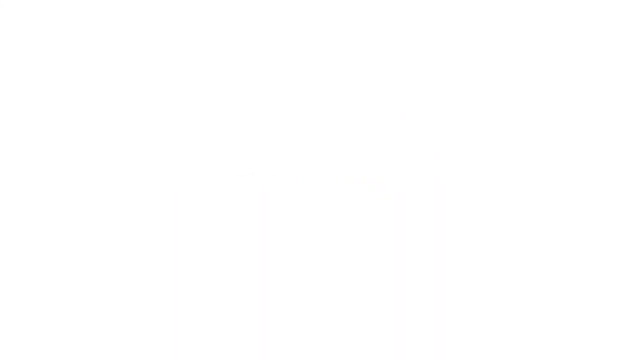 In today's video, we're going to look at the difference between scalar and vector quantities, which can also be called scalars and vectors. Scalars are physical quantities that only have a magnitude but no direction, And remember, magnitude is just another way of saying size, and so it can be measured with a numerical. 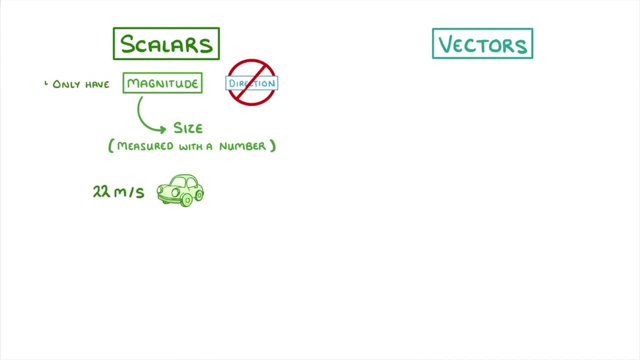 value. For example, if a car travels at 22 metres per second, 22 would be the magnitude of the speed, And because speed by itself doesn't have a direction, we consider it a scalar quantity. Other scalar quantities include things like distance, mass, temperature and time, although there are loads more. 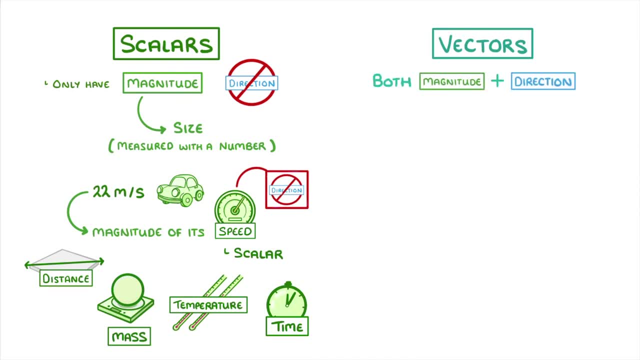 Vectors, on the other hand, have both a magnitude and a direction. These include things like velocity, displacement, acceleration, force and momentum. We take a closer look at each of these quantities in other videos, though, so don't worry if you're not sure what. 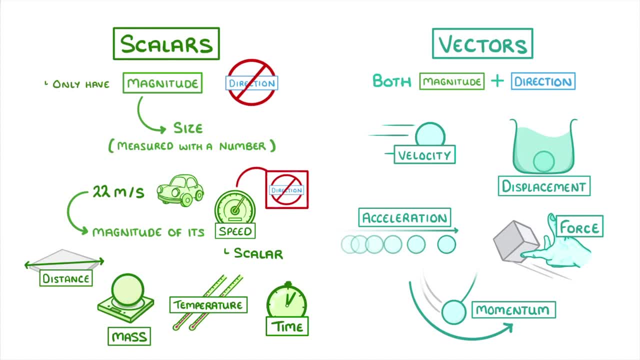 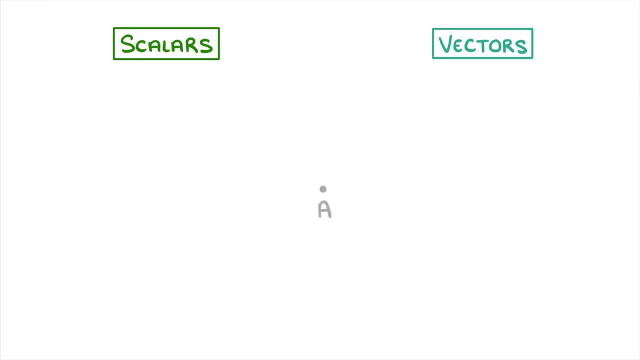 any of them are. just yet, To help you understand the difference between scalars and vectors, imagine you start with this point A and you walk a distance of 3 kilometres. Depending on which way you set off, you could end up anywhere on the circumference of this circle. This is because 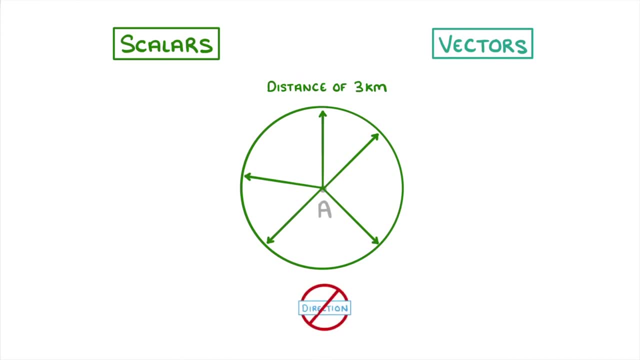 distance doesn't actually give us any idea of the direction, which is why it's a scalar quantity. However, if you'd started at A and then told us that you walked 3 kilometres east, we'd know exactly where you ended up, because you gave 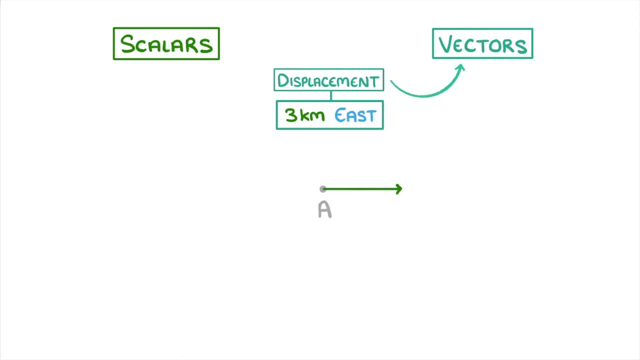 the exact displacement, which is a vector quantity, because it has both a magnitude of 3 kilometres and the direction of east. In order to represent vectors, we use arrows with the length of the arrow indicating the magnitude of the vector and which way it's pointing, indicating the direction, So 4 kilometres.